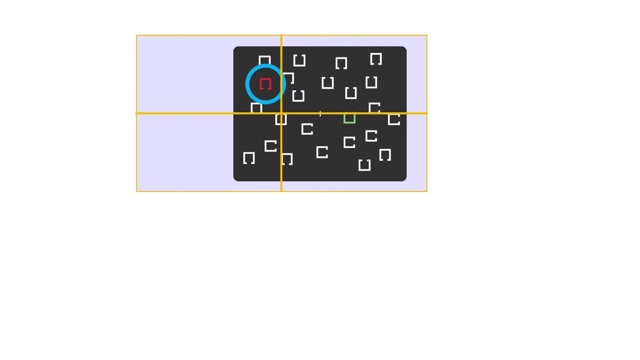 shift their gaze to the left side of the display before the stimuli appear. As a result, most of the stimuli will be in the right visual field, which would give you a lateralized ERP. It would be hard to tell the difference between this sensory lateralization and the N2PC. 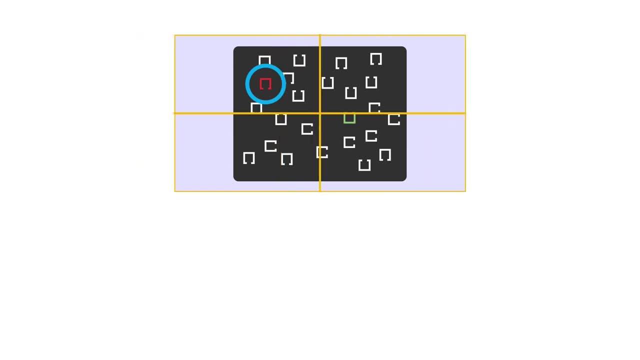 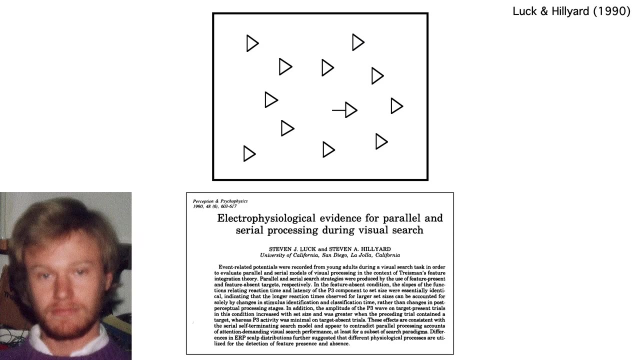 So we need to make sure that subjects keep their eyes on the fixation point or we end up with a physical stimulus confound. Here's another physical stimulus confound. This is actually the experiment where I originally discovered the N2PC when I was in grad school. 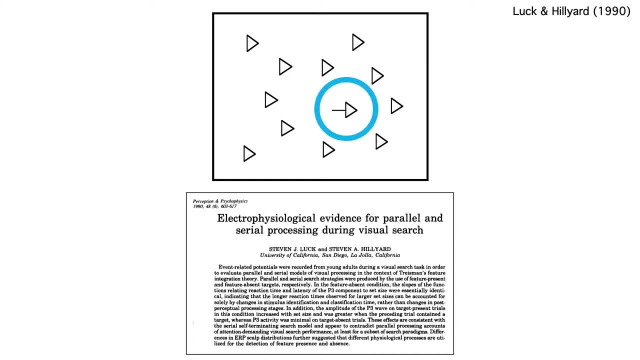 back when I had more hair. The target was the triangle with the horizontal line and subjects pressed one of two buttons to indicate whether the target was present or absent. The problem with this design is that the contralateral and ipsilateral sides of the display were physically different. The contra side had a horizontal line. 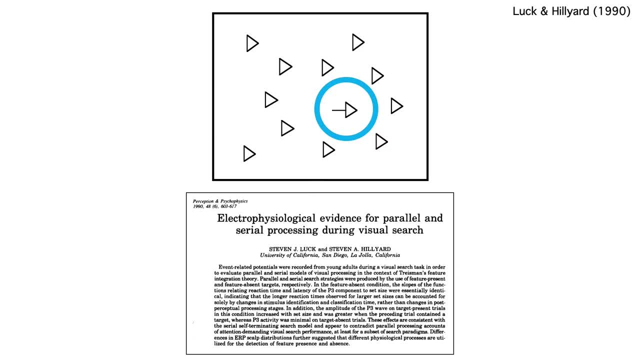 and the ipsi side didn't. This might have been responsible for the contralateral negativity that I saw from 200 to 300 milliseconds. We later ruled out that possibility, but it was a flaw in the original design. Now we typically use this kind of design We have. 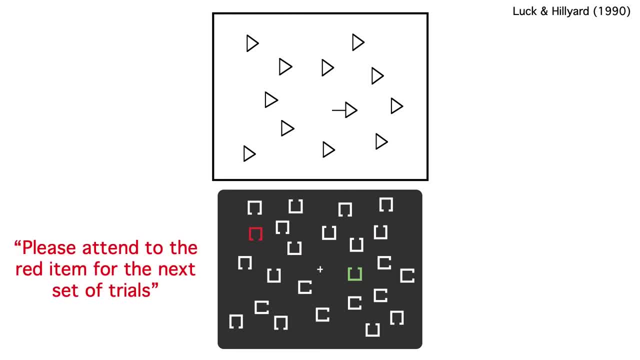 a red item on one side and a green item on the other. Subjects are instructed to attend to the red item for some trial blocks and to the green item for others. The stimulus positions vary randomly from trial to trial. The stimulus positions vary randomly from trial to trial. The stimulus 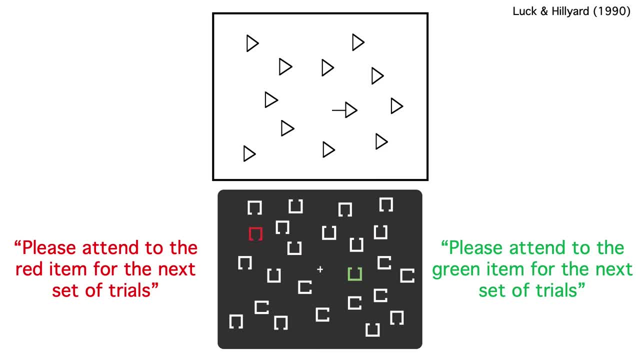 positions vary randomly from trial to trial, so subjects can't predict which side will contain the target before the array is presented. This design allows us to compare the same physical stimuli while varying whether the subject is attending to the left side or the right side. 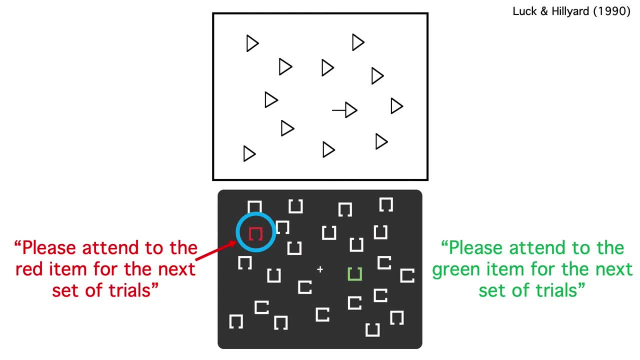 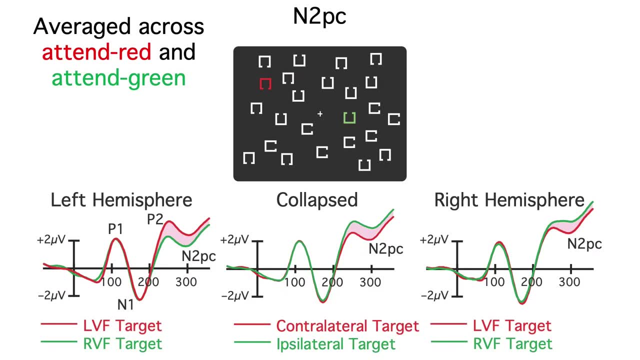 For this array, subjects will shift their attention to the left side in the attend red blocks and to the right side in the attend green blocks. Same stimulus but different directions of attention. Then we look at the data contralateral versus ipsilateral to the attended side collapsed across attend red and attend green blocks. 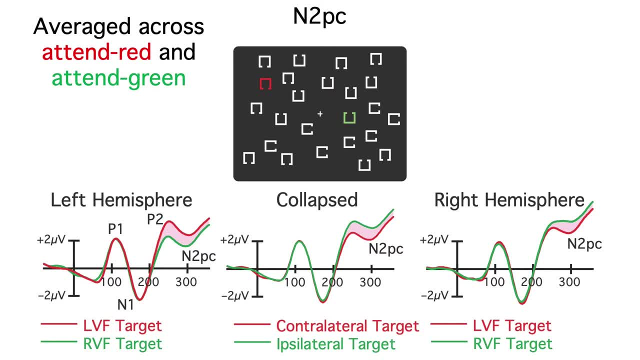 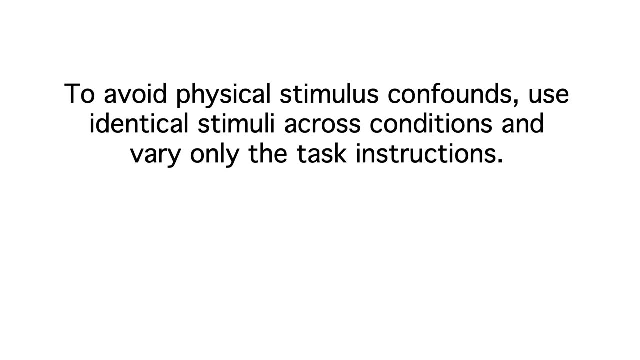 This allows us to be sure that the difference in voltage between contra and ipsi electrodes reflects the side being attended, not a difference in the physical stimuli between the two sides. This exemplifies an important rule To avoid physical stimulus confounds: use identical stimuli across conditions and vary only the task instructions. 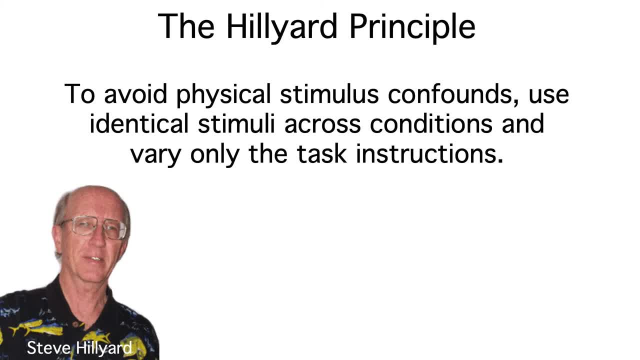 I call this the Hilliard principle because it was drilled into me when I was a grad student in Steve Hilliard's lab back in a previous century. Steve was incredibly careful about experimental design and as a result he made huge scientific contributions using ERPs.